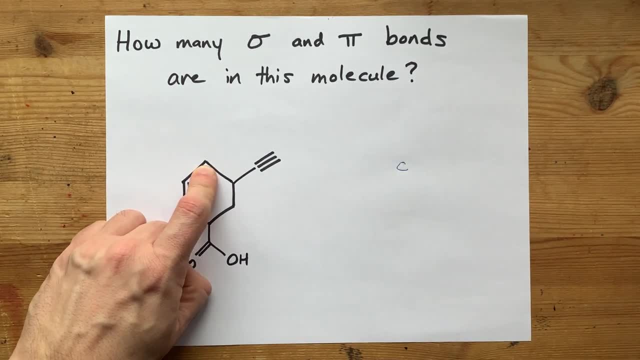 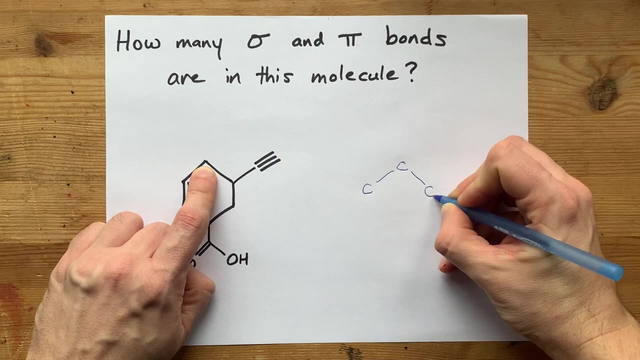 at the top here. I'm going to put a C there. Now. I don't have any bonds yet, so let's not get excited. I do have a single bond to this carbon down here and a single bond to this carbon down here. The first bond between any two atoms is sigma, so I already have one, two sigma bond. 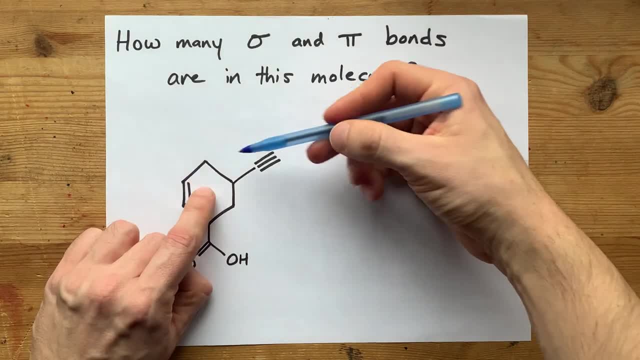 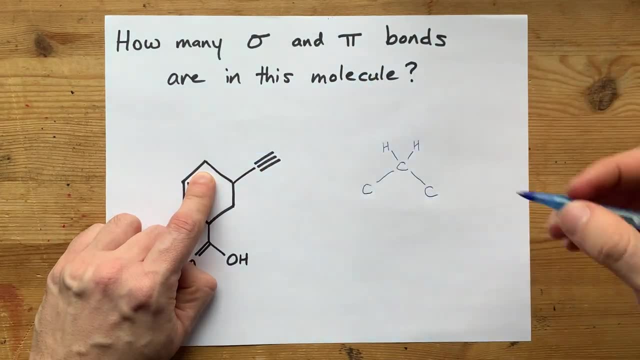 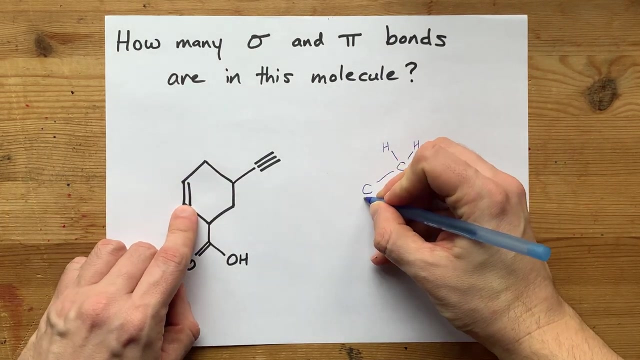 But carbon atoms need four bonds total. so what gives with that one? Well, the answer is that there's a bond to a hydrogen and another hydrogen, both of which are not shown on this diagram. So that's four sigma bonds total. so far. I'm going to proceed this way. There's a sigma bond. 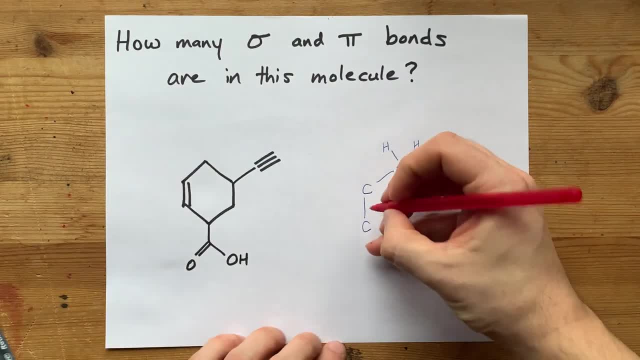 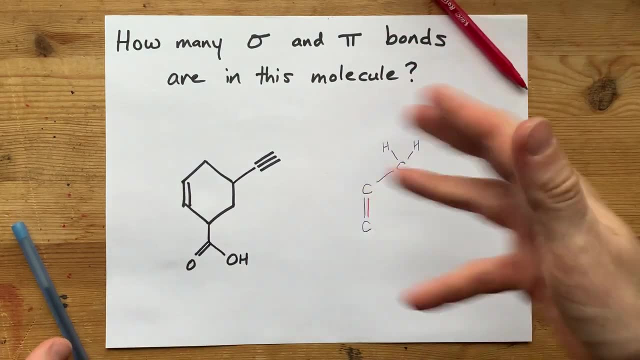 between this carbon and that carbon. but then the second bond between those two is pi. I'm going to put it in red. I do expect four of those pi bonds by the time that we're done with this diagram, But I guess when I catch that last one I'll just put it on the side And I'm gonna think that. 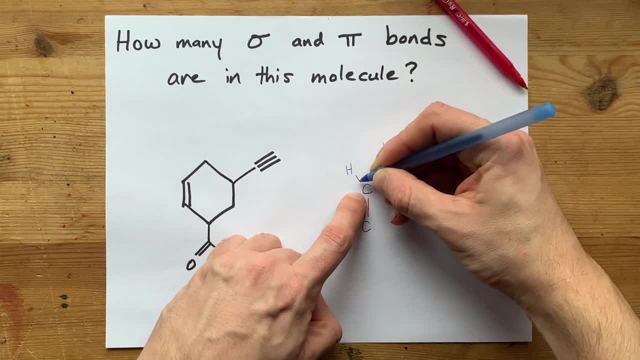 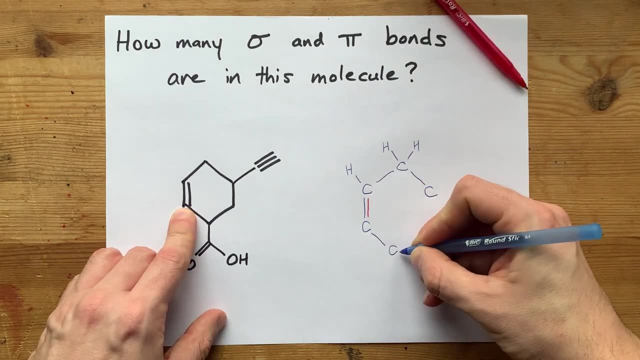 let's clear of that last one, because that's fine. Un gente is Hil, WHOis nucleic. I'm just gonna put the firstLet's say: And now let's do this again. Alright, let's let's show again that if I have a four bond with pi and plus BeR. 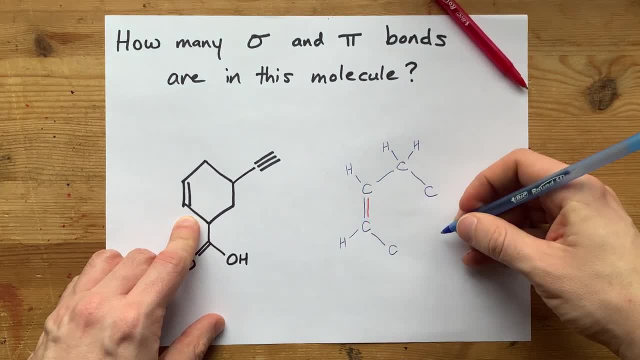 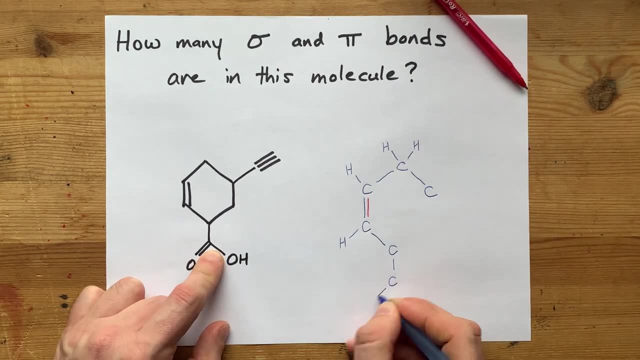 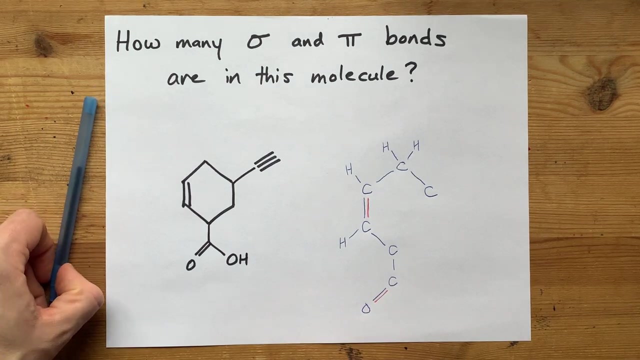 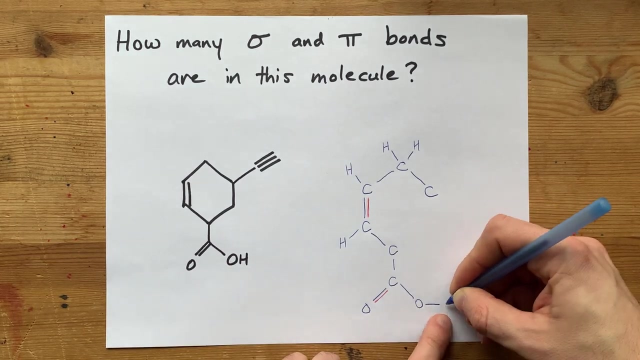 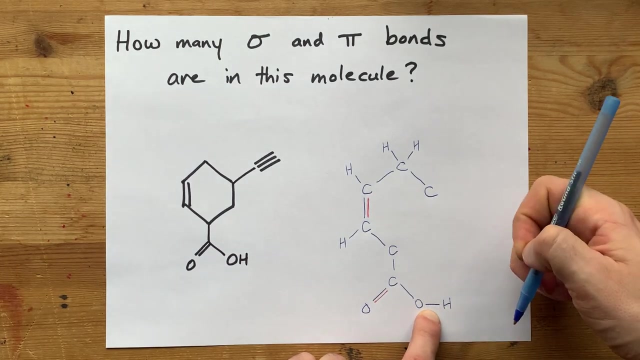 an oct. no wait, double bonded. The second bond between the two is pi. Now that was bonded to an oxygen and that oxygen was bonded to hydrogen. I'm going to explicitly show that bond with a single line here, to show that it is an extra sigma bond in the molecule. 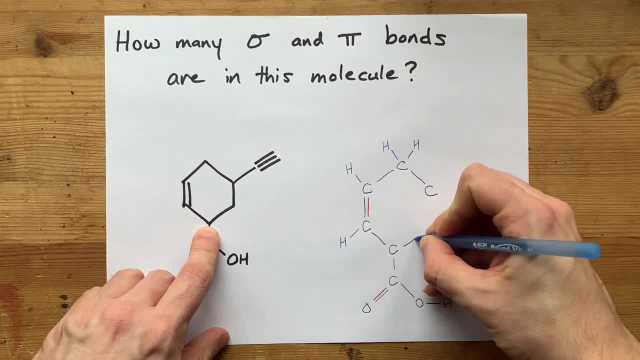 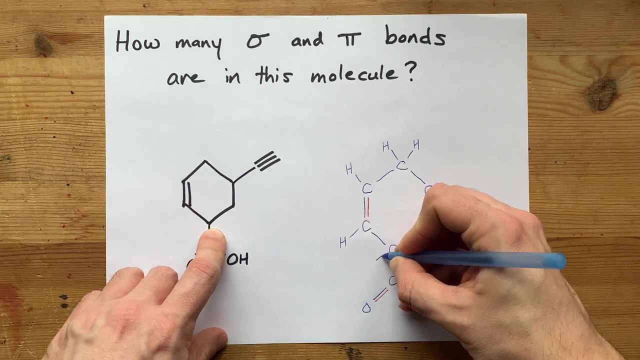 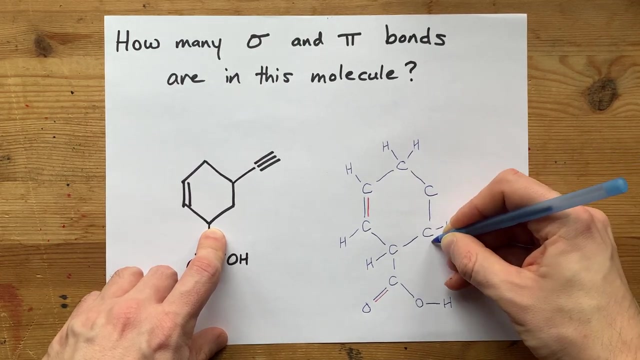 Now I'm done with this substituent here, so I'm going to come back up Carbon. Now that carbon has one, two, three things bonded to it, so I need a fourth. There's the hydrogen that was not shown. That carbon was single. bonded to that carbon, It had two hydrogens that weren't shown. 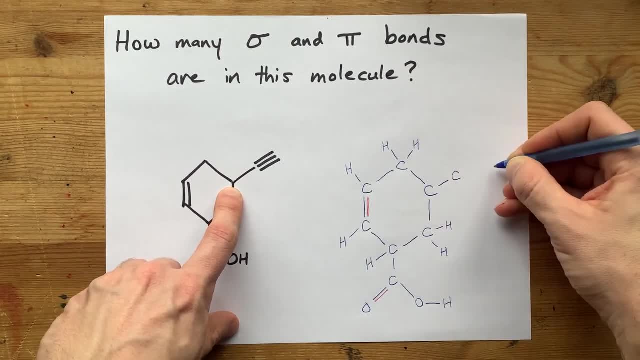 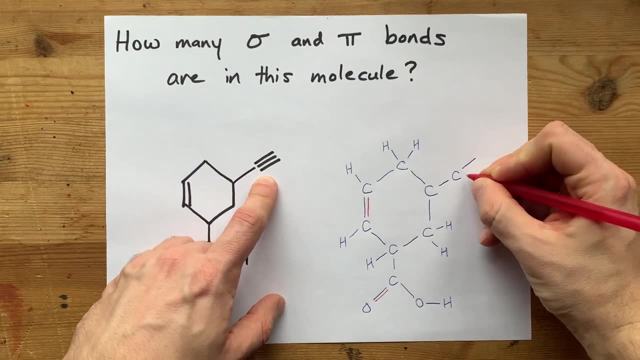 That carbon was single bonded to another carbon and then it was triple bonded to the next carbon in the chain. The first bond between the two is sigma, The next two are pi. Oh, look one, two red lines for the two pi bonds.